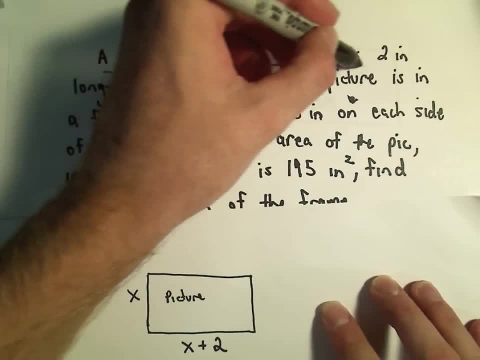 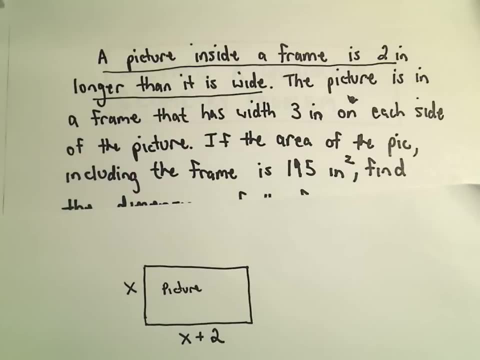 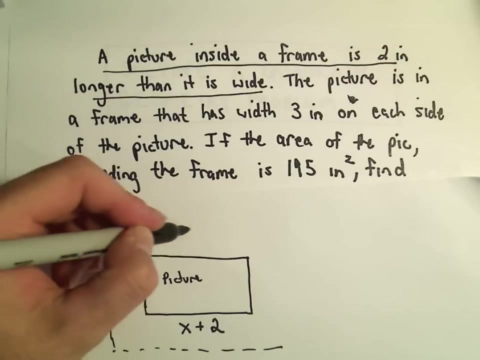 So we're kind of using this first sentence here, So it's 2 inches longer than it is wide. But we also know that there's a little line here, So we're going to draw a little picture frame around this. 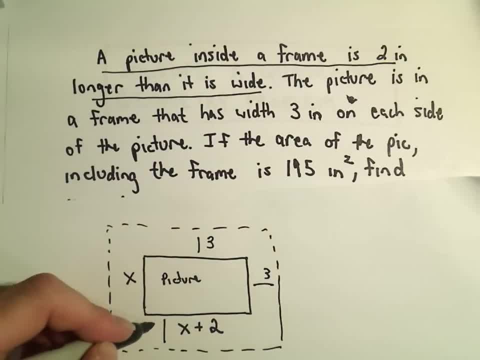 And we know that that is 3 inches on each side. Okay, so, if you think about it, since we know that the original we'll call this the length, Since that was x plus 2, since there's 3 inches on one side and another 3 inches on the other side. 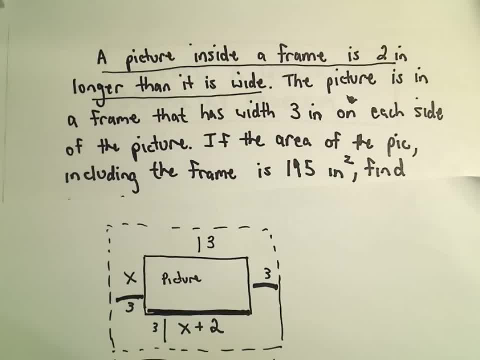 that means the picture frame is going to have a length of x plus 2.. So it's going to have a length of x plus 8.. And likewise, since we said its width was x, since there's 3 inches above it and 3 inches below it. 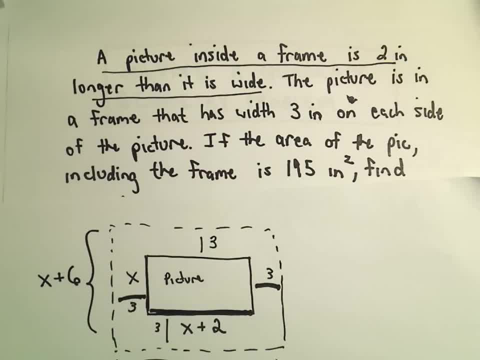 the other dimensions of the picture frame would have to be this value: x plus 6.. Okay, so we know. though we know the total area of this picture, including the frame, is 195.. Well, the area would simply be the length times the width. 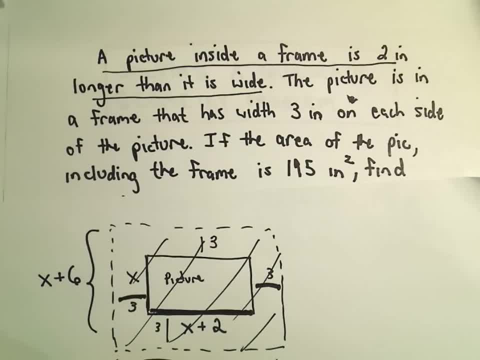 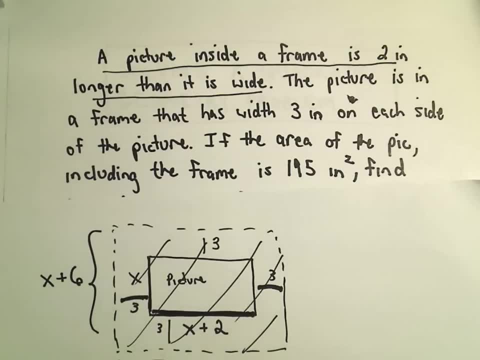 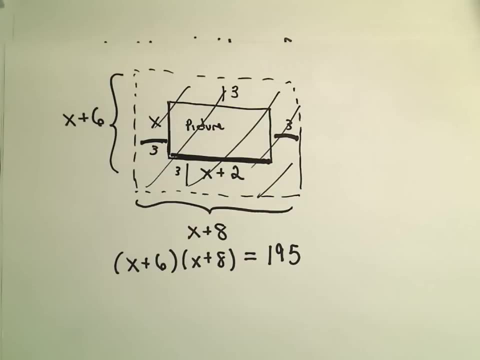 So we would have to take x plus 6 times x plus 8, and we'll simply set that equal to 195.. And now we have our little quadratic equation that we're going to have to solve. Okay, so what I'm going to do is multiply out the left side. 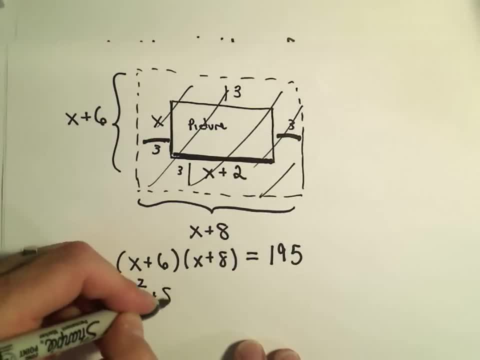 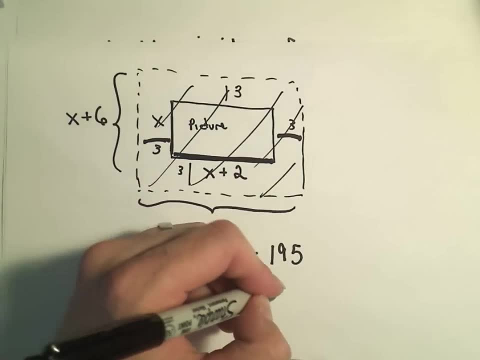 So x times x would be x squared, We would get a positive 8x. On the inside we'll get a positive 6x. 6 times 8 is 48. And that's going to equal 195.. 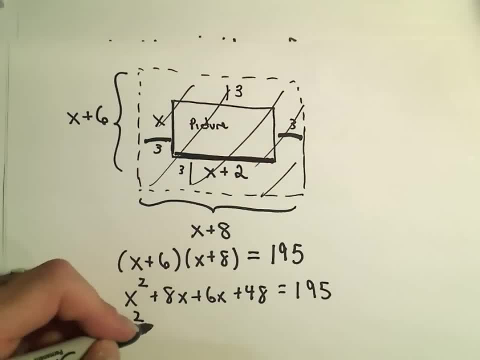 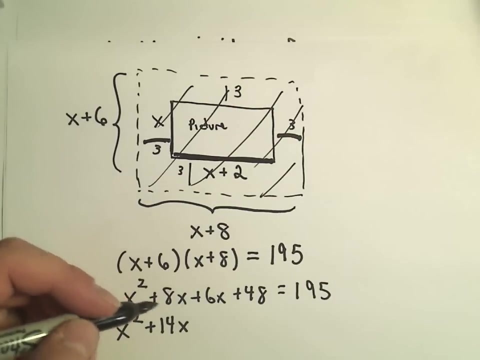 So okay, so we have x squared. 8x plus 6x is going to give us 14x. If we take 48 and subtract away 195 from both sides, that's going to give us the value negative. 147 equals to 0.. 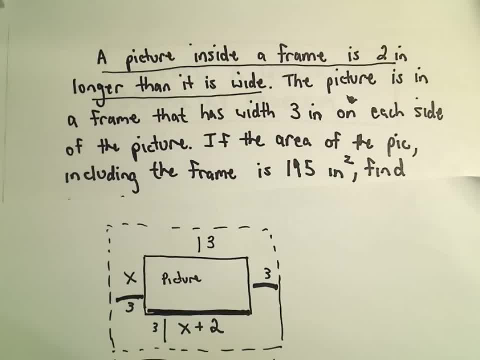 that means the picture frame is going to have a length of x plus 2.. So it's going to have a length of x plus 8.. And likewise, since we said its width was x, since there's 3 inches above it and 3 inches below it. 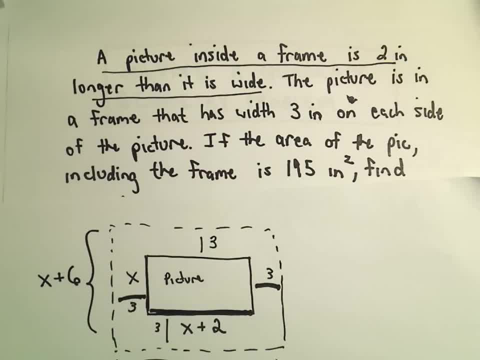 the other dimensions of the picture frame would have to be this value: x plus 6.. Okay, so we know. though we know the total area of this picture, including the frame, is 195.. Well, the area would simply be the length times the width. 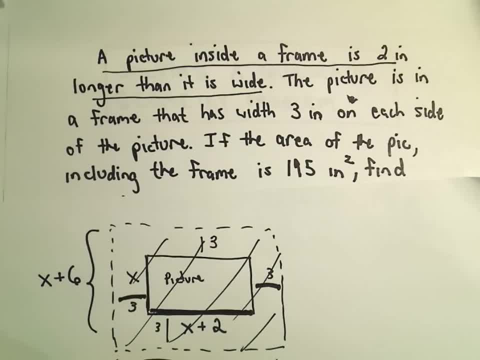 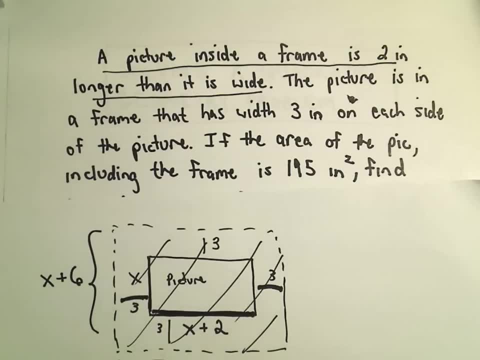 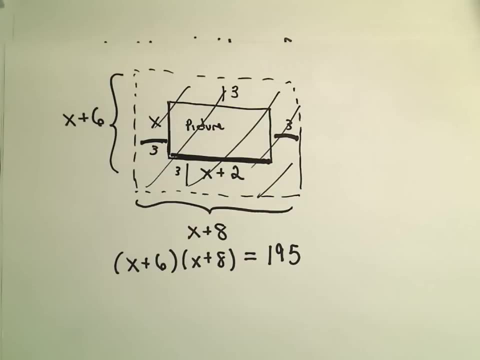 So we would have to take x plus 6 times x plus 8, and we'll simply set that equal to 195.. And now we have our little quadratic equation that we're going to have to solve. Okay, so what I'm going to do is multiply out the left side. 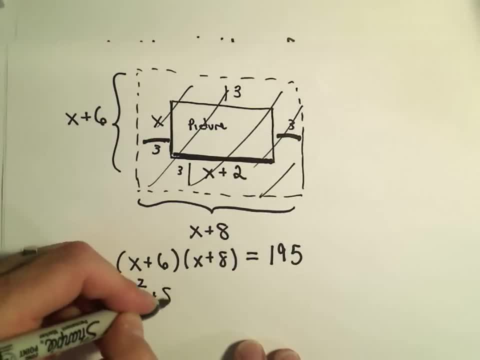 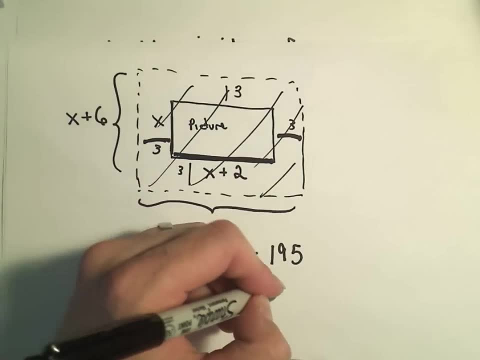 So x times x would be x squared, We would get a positive 8x. On the inside we'll get a positive 6x. 6 times 8 is 48. And that's going to equal 195.. 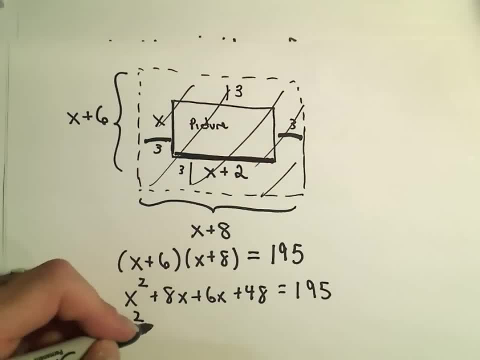 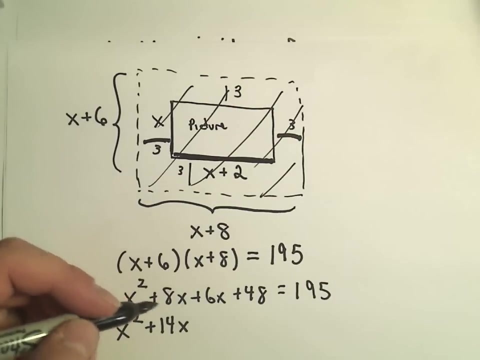 So okay, so we have x squared. 8x plus 6x is going to give us 14x. If we take 48 and subtract away 195 from both sides, that's going to give us the value negative. 147 equals to 0.. 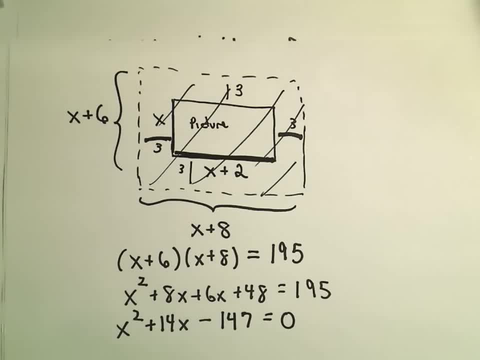 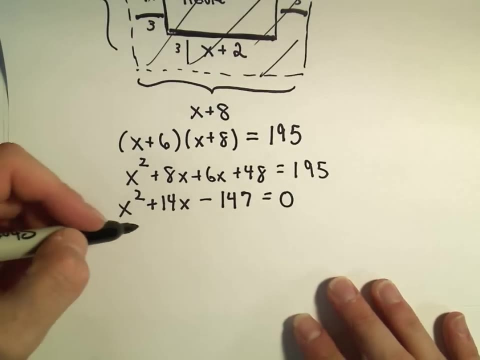 And now there's a couple of different things that you could do here. You could either try to, You could either use the quadratic formula. Maybe you could try to factor it here a little bit. I think it's definitely going to factor, if my math here is correct. 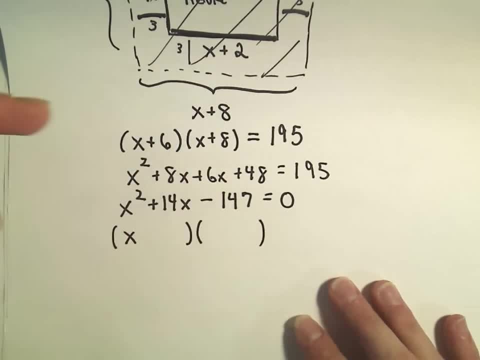 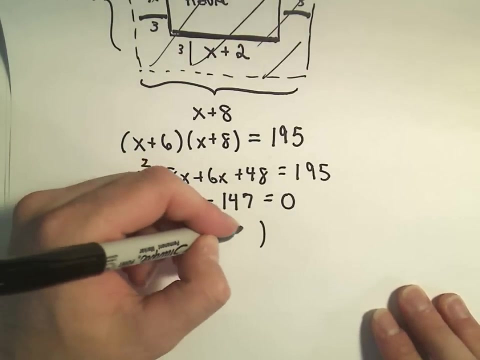 So I believe this actually factors here. So we're looking again for two numbers that multiply to negative 147 but add up to positive 14.. Well, let's see here: What if we use- How about negative 7? and what if we use positive 21?? 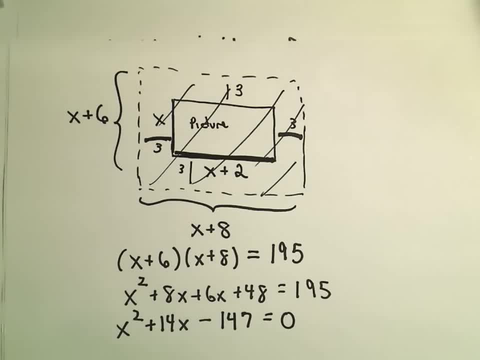 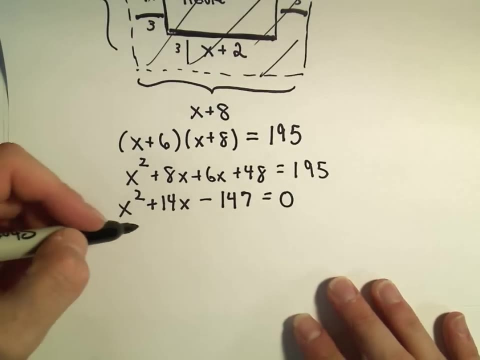 And now there's a couple of different things that you could do here. You could either try to, You could either use the quadratic formula. Maybe you could try to factor it here a little bit. I think it's definitely going to factor, if my math here is correct. 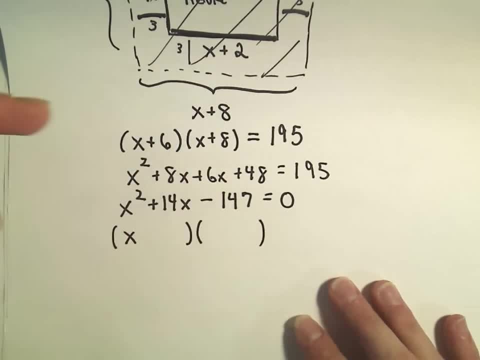 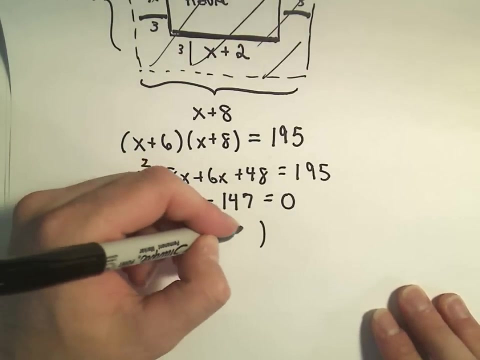 So I believe this actually factors here. So we're looking again for two numbers that multiply to negative 147 but add up to positive 14.. Well, let's see here: What if we use- How about negative 7? and what if we use positive 21?? 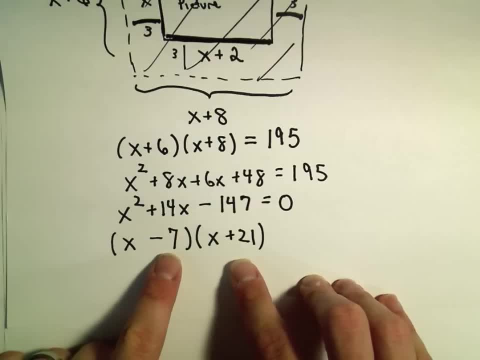 So I'm pretty good with arithmetic. here You can check that if you take negative 7 times positive 21, you'll get negative 147.. If you add negative 7 and positive 21,, hey, that does give you positive 14.. 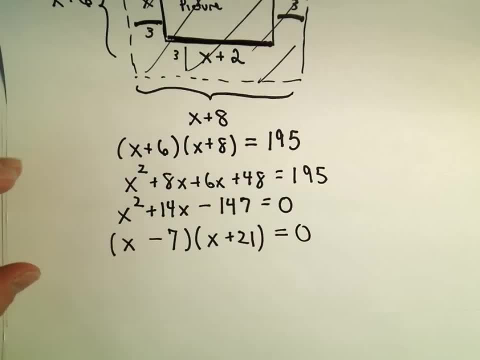 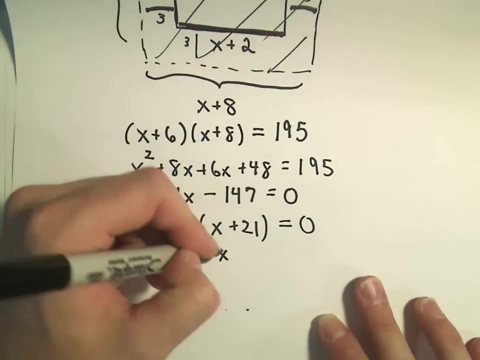 So this is a correct factorization. You know, again, if you feel like this would be kind of a step that you're not sure about, simply I would just use the quadratic formula and find the solutions that way. Okay, so at this point we just set each part equal to 0.. 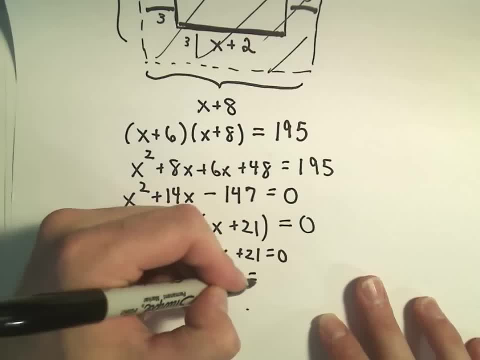 Okay, so if we solve the first part, we'll get x equals 7.. The other part, we'll get x equals negative 21.. Since x has to do with, you know, the width and inches, it doesn't make sense for it to be negative 21 at all. 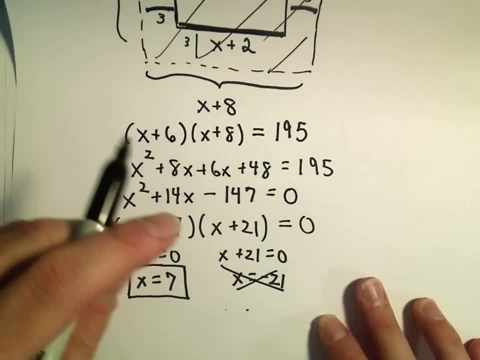 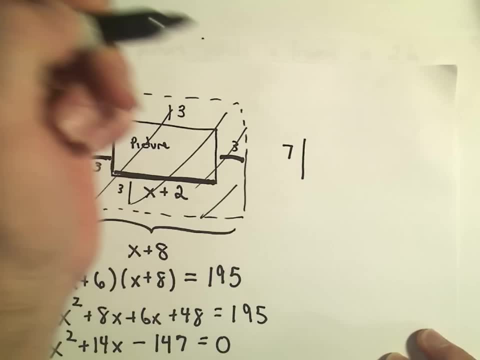 So the only solution that makes sense here is the value x equals 7.. So now we can go back. So the original dimensions of the picture: it was 7 wide, And since it was 2 inches longer it would have to be. 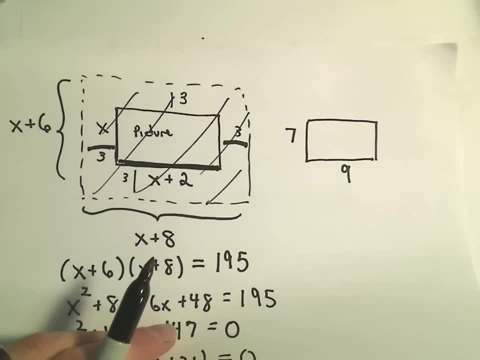 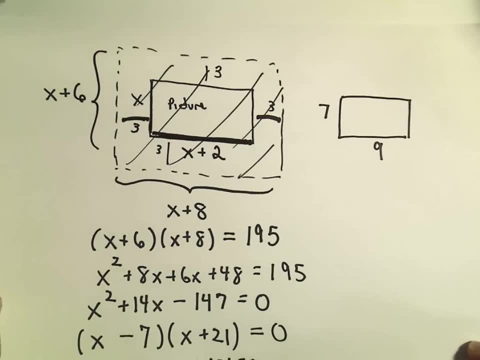 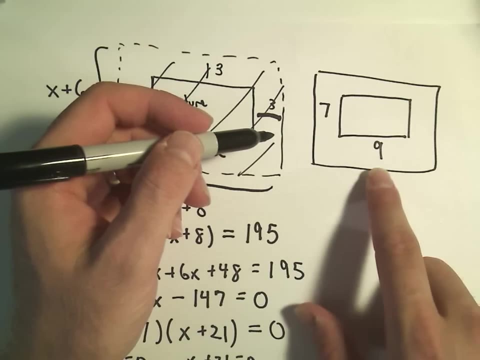 The original picture would have to be a 7 by 9.. 7 inches by 9 inches would be the original size of the picture. I think the original problem asked for the dimensions of the frame. So if we actually look at the frame, since we have to add on 3 inches to each side, 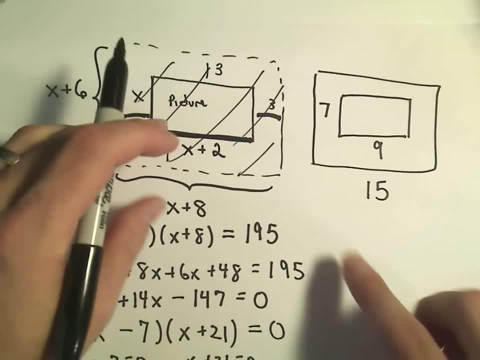 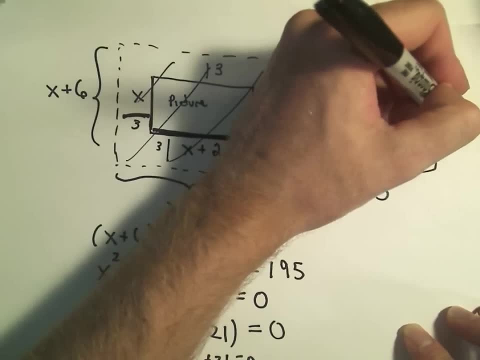 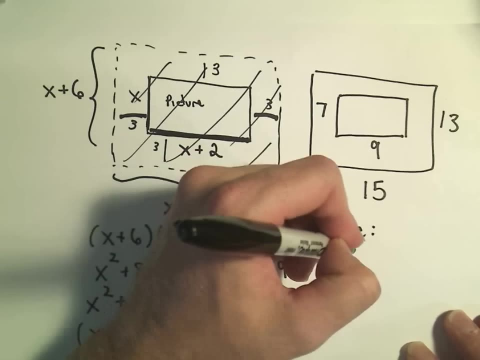 we would get 9 plus 6.. So the frame would have a length of 15.. We would also have to add 6 to the width. So if we add 6 to that, we'll get 13.. So it looks to me like the dimensions of the frame we could say is 13 inches by 15 inches.